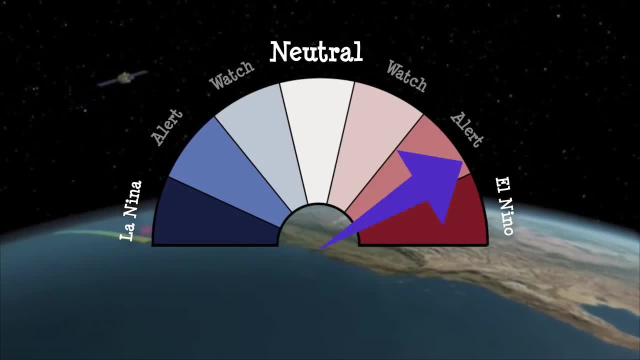 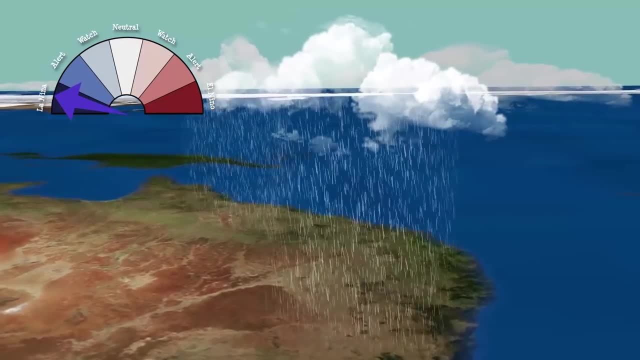 the three phases of ENSO Neutral, El Niño and La Niña. A La Niña event tends to bring above average rainfall to eastern Australia. During an El Niño event, there is a greater chance of drought and bushfires. 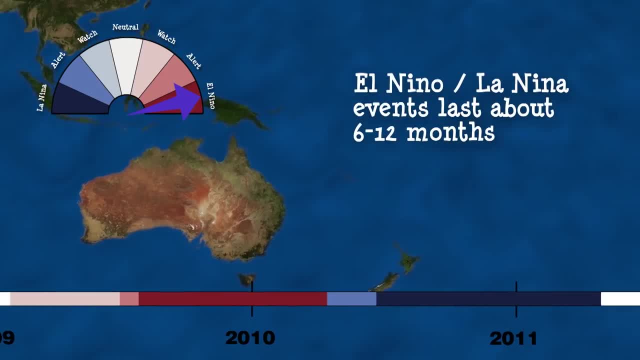 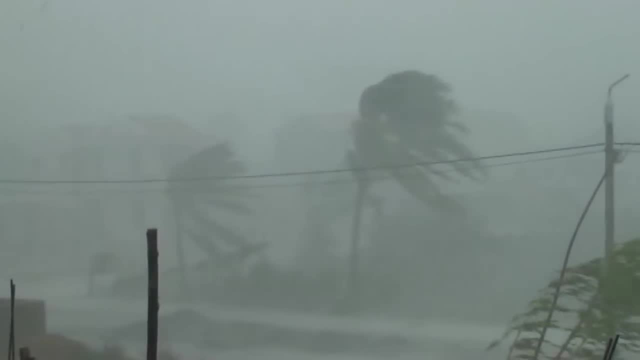 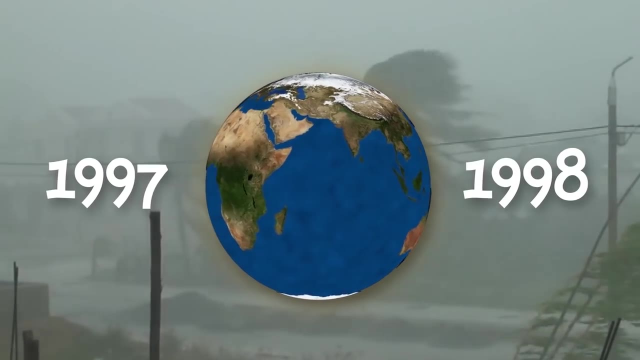 Each El Niño and La Niña event lasts about 6 to 12 months. It takes on average four years to cycle from El Niño to La Niña and back again, But no two El Niños are the same. The strong 1997-98 El Niño impacted every continent in the world, causing widespread 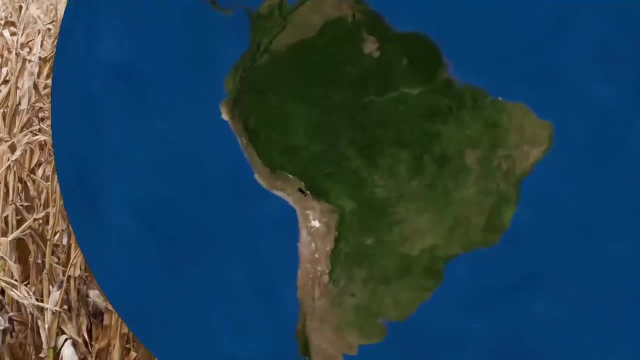 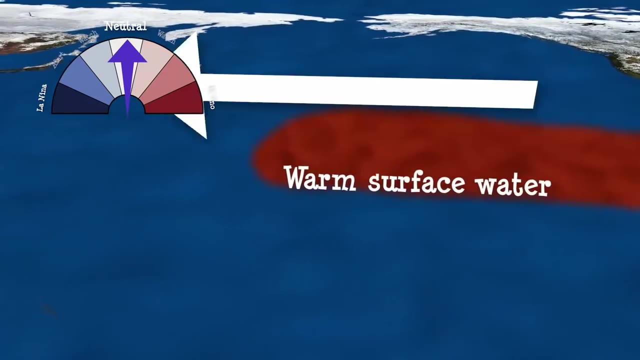 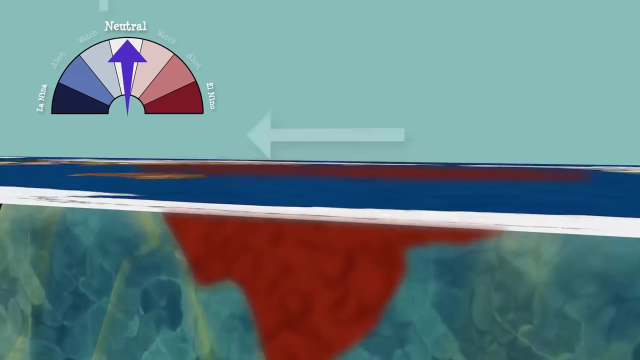 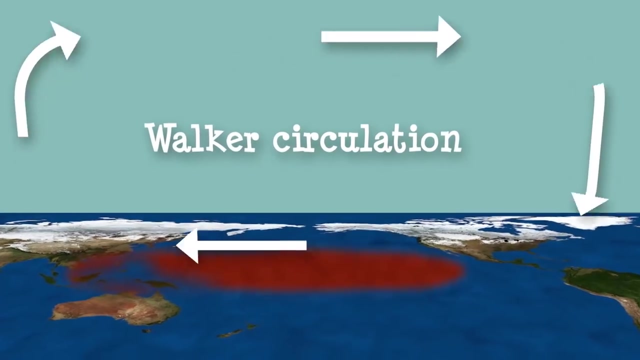 devastation worldwide. This story begins in the eastern Pacific. Here, trade winds blowing from east to west push warm surface waters across the planet, piling up warm water in the western Pacific. Above the ocean, warm air rises, driving atmospheric circulation into the prickly waters En primer tipo. constant stream of water at low tide creates. 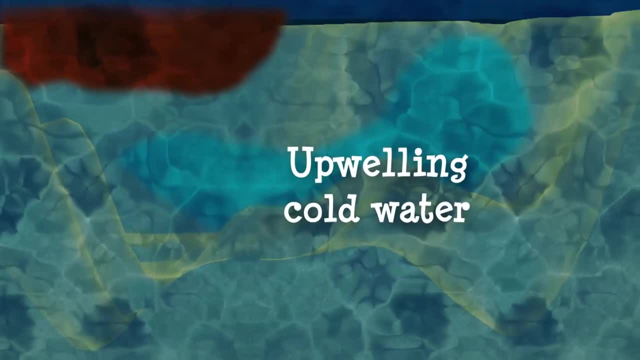 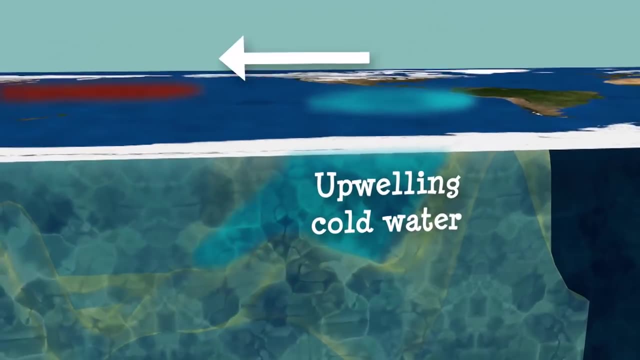 a reaction, But that is far out of the reach of any tropical sea. Cold, nutrient rich waters up well in the coastal ocean, replacing the warm water pushed away by the trade winds Like an athlete pumping iron. the La Niña is the muscled-up version. 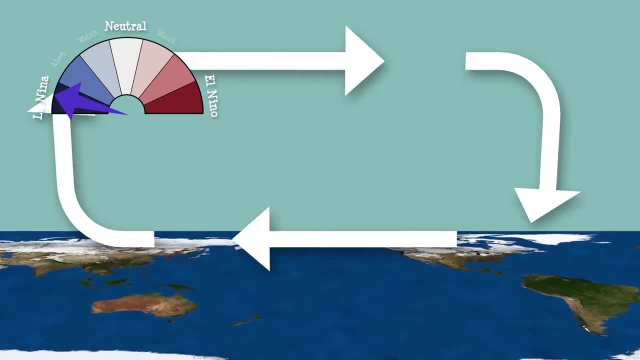 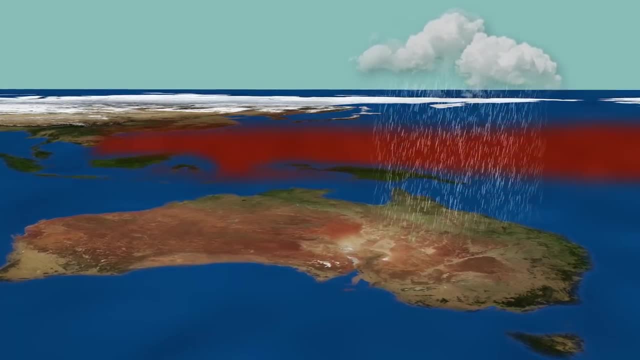 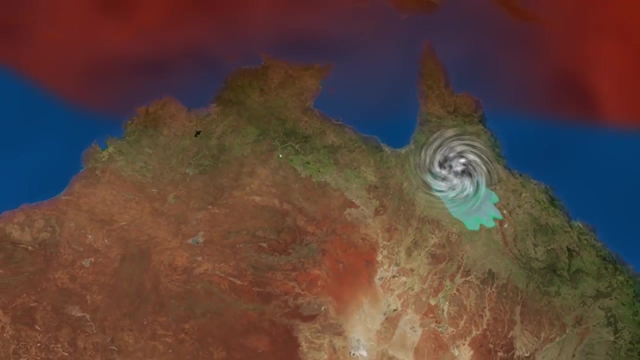 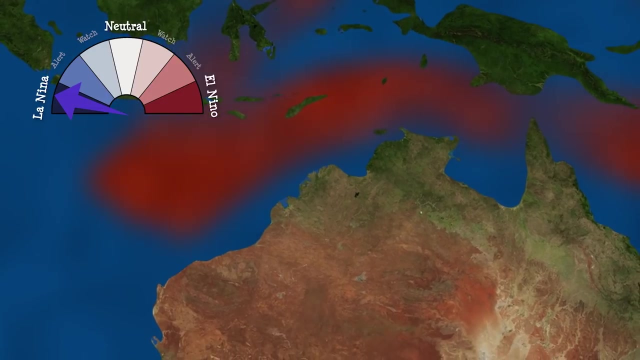 of the neutral phase, Trade winds become strong and more warm water builds up in the west Pacific. The excess of warm water increases evaporation and precipitation, A warming of causing floods and forming tropical cyclones off the northeastern Australian coast. This warm water escapes through the gap between Indonesia and Australia. 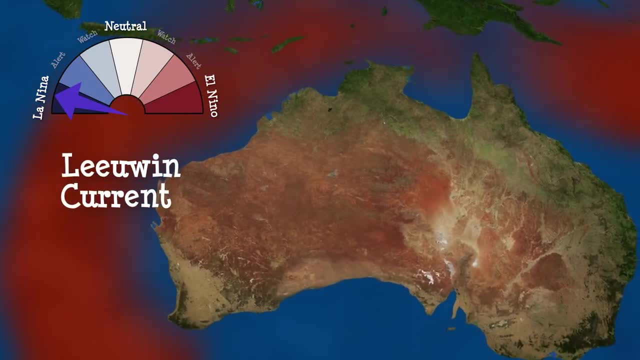 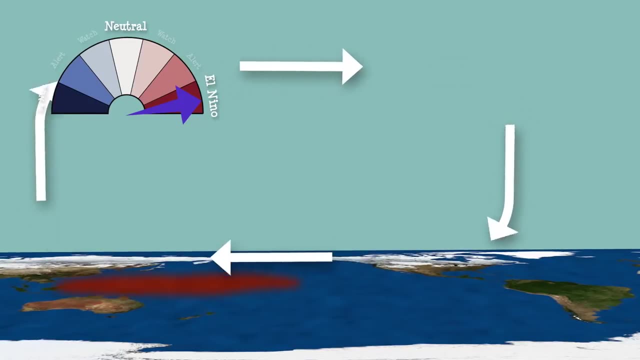 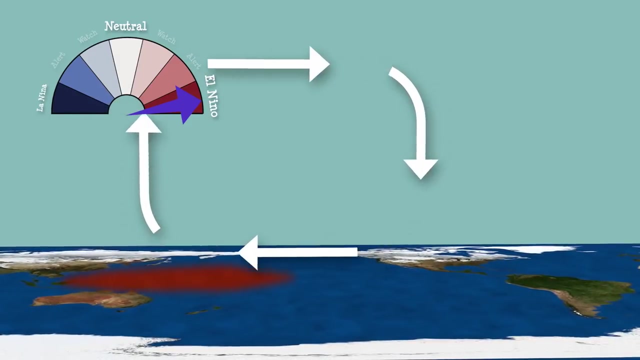 to supercharge the Lewin Current, a 5,500 kilometre long flow of warm waters along the western Australian coast. But like an athlete, the winds can't keep pumping at this speed forever. Sometimes the winds weaken and warm water sloshes back across the ocean to the East Pacific. 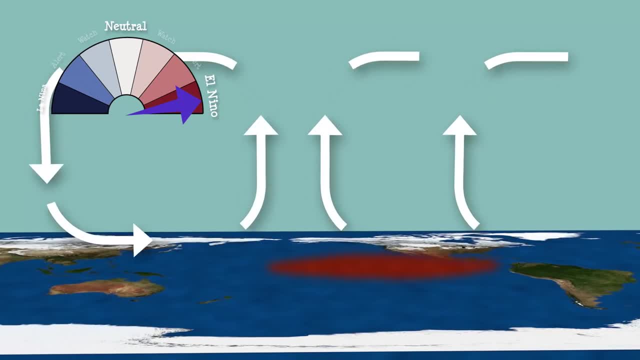 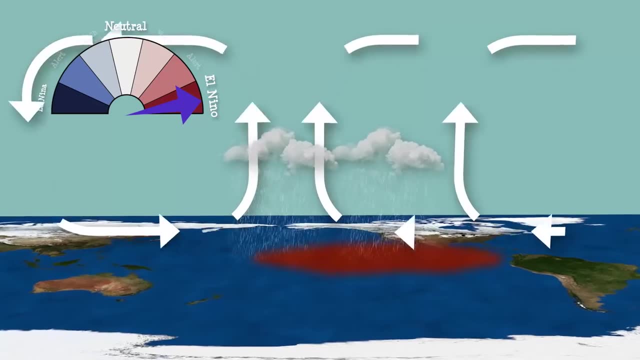 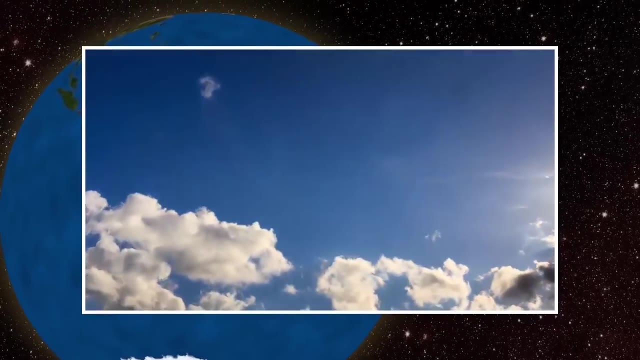 The Walker Circulation breaks down, weakening or even reversing the trade winds, Warming of the Eastern Pacific accelerates, setting off a feedback loop that keeps most of the rain-producing evaporation in the middle of the Pacific, Due to the movement to the east of warm surface waters.